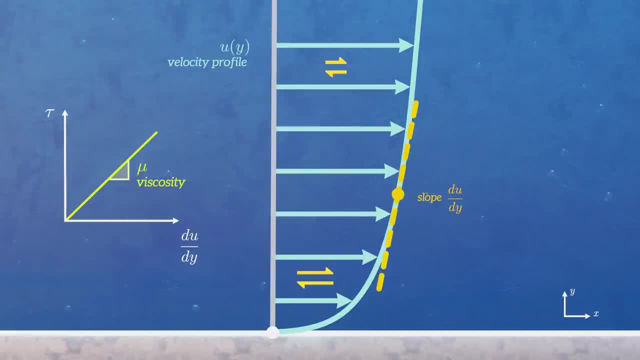 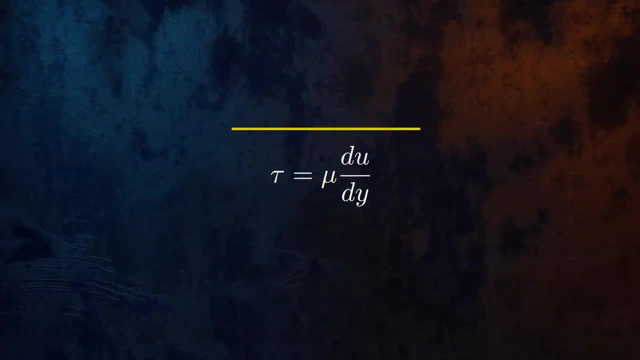 smoothing out differences in velocity by increasing the shear stresses in proportion with the velocity gradient. We can express the linear relationship using this equation. This is called Newton's law of gravity, and fluids that obey it are said to be Newtonian. It describes how easily a fluid will. 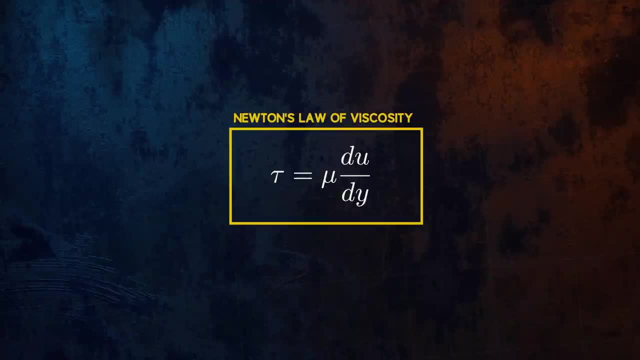 flow. The viscosity mu is sometimes called the dynamic viscosity, as this differentiates it from the kinematic viscosity, which is the dynamic viscosity divided by the fluid density. Let's look at how a small fluid element like this one will deform as it flows. 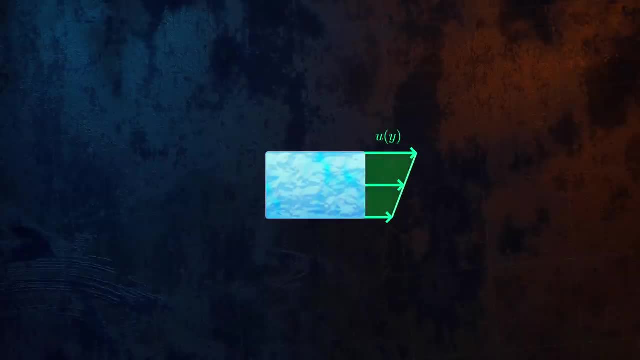 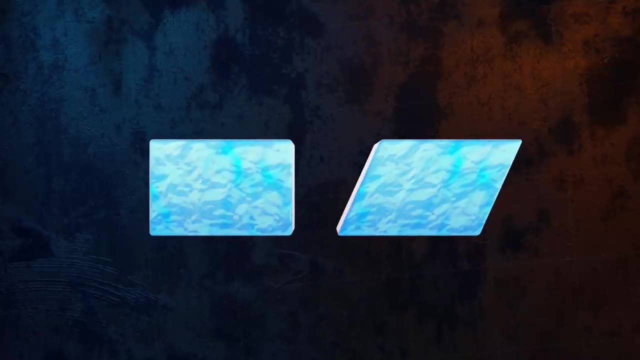 If du over dy is positive, the upper surface will move faster than the lower surface, and so over a time period, delta t- the upper surface will travel further by a distance equal to delta u times delta t. This generates a shear strain. 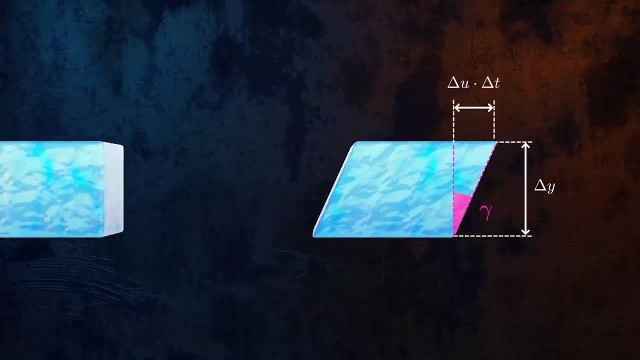 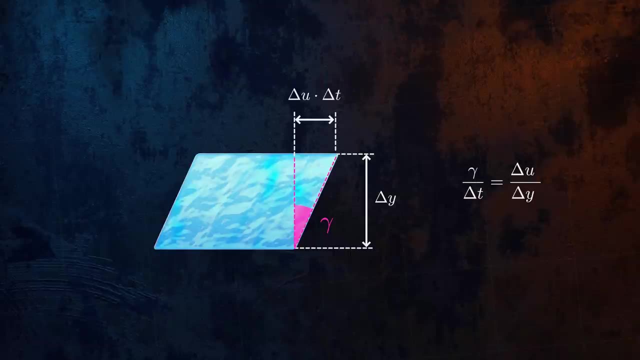 that we can calculate using trigonometry and the small angle approximation. By rearranging, we can see that the slope of the velocity profile is equivalent to the rate at which the shear strain is applied. So now we can write Newton's law of viscosity in a different. 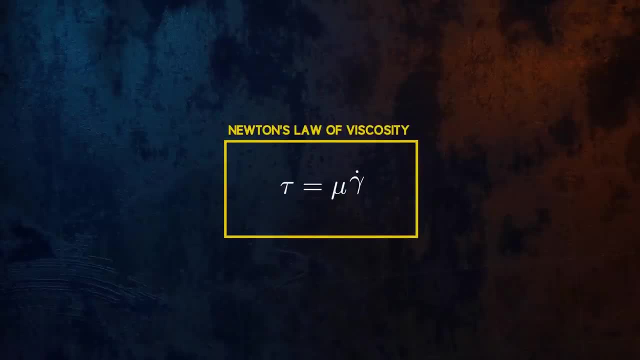 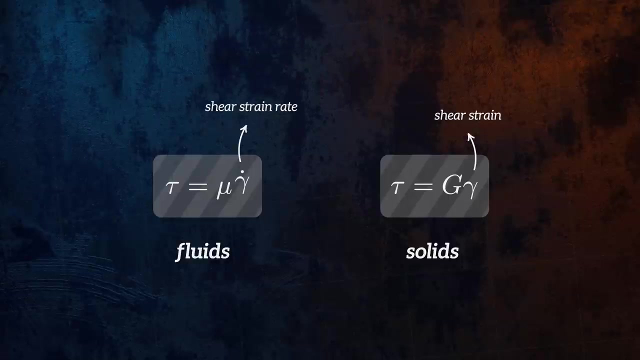 form like this. This looks a lot like Hooke's law for shear that we see in solids, except instead of being a function of the strain, the shear stress is a function of the rate at which the strain is applied. This makes sense if we consider how solids and fluids respond to applied shear forces. 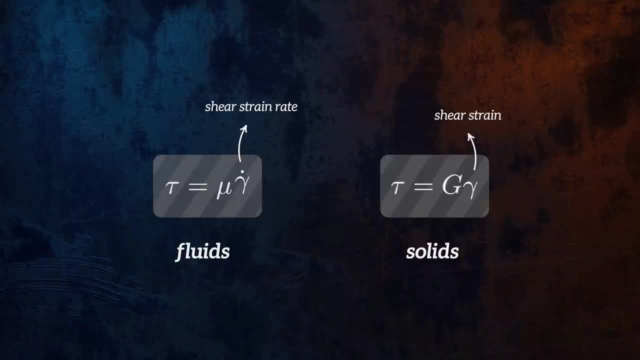 The shear stress is a function of the rate at which the strain changes over time. whereas fluids respond by deforming continuously, They flow for as long as the shear force is applied. This is why, for fluids, the shear stress is a function of the rate at which strain changes. 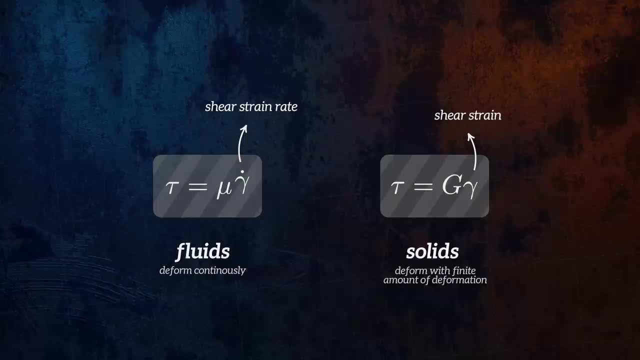 over time, instead of being a function of the shear strain itself, like it is for solids. If we do some quick dimensional analysis on Newton's law of viscosity, we can see that the dynamic viscosity has been increased by a significant percentage. This is because the shear stress is. 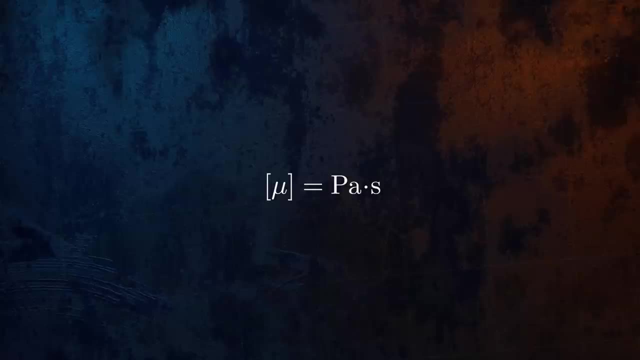 a function of the rate at which the strain changes over time. The kinetic viscosity has units of Pascal seconds and the kinematic viscosity has units of meters squared per second. The poise and stokes are other units for the dynamic and kinematic viscosities. 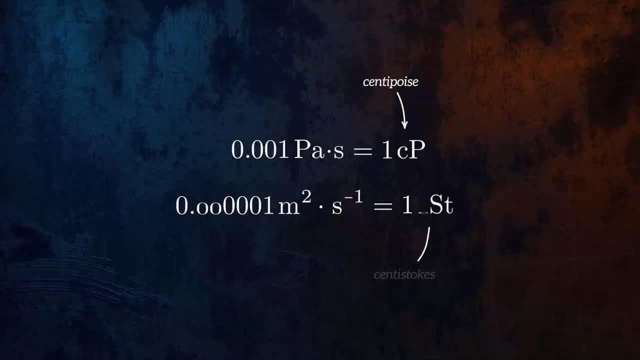 although they are often expressed as centipoise and centistokes. The centipoise unit is particularly convenient because at room temperature the viscosity of water is equal to one centipoise. Typical engine oil at room temperature has a viscosity of one centipoise. 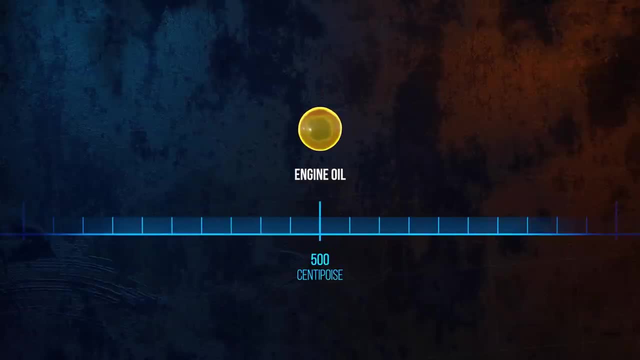 Typical oil at room temperature has a viscosity of around 500 centipoise, so is 500 times more viscous than water. The viscosity of honey is 10,000 centipoise and if we keep going we get to fluids that are so viscous they appear to be solid. 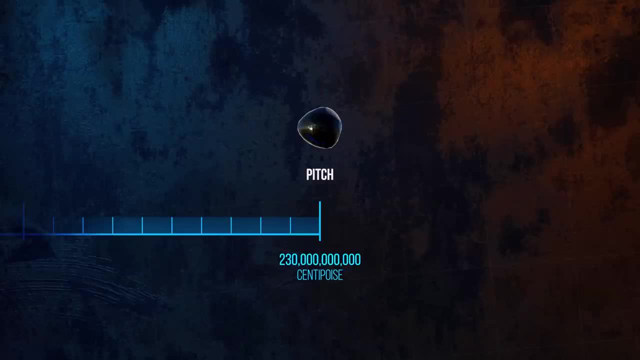 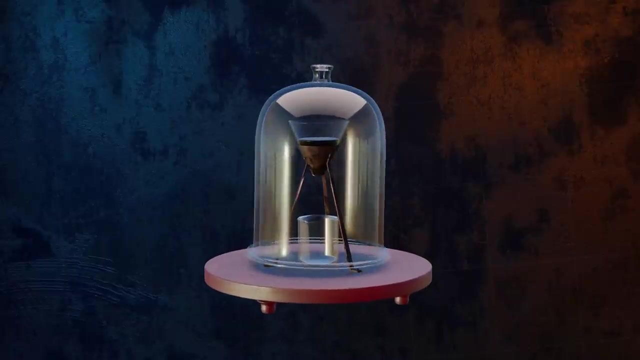 Pitch is a thick, tar-like fluid that has extremely high viscosity, as is famously demonstrated by the pitch drop experiment. In 1927 at the University of Queensland, heated pitch was added to a funnel and once it cooled it was allowed to drop into a beaker placed below it. 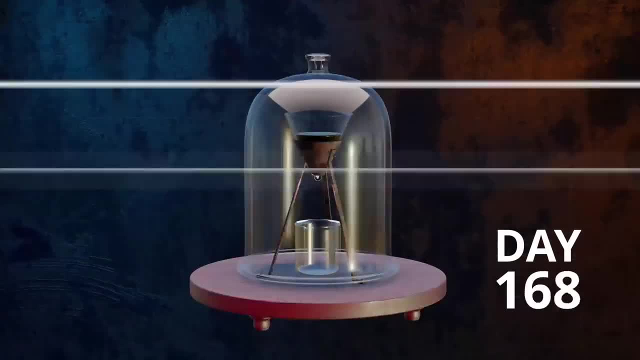 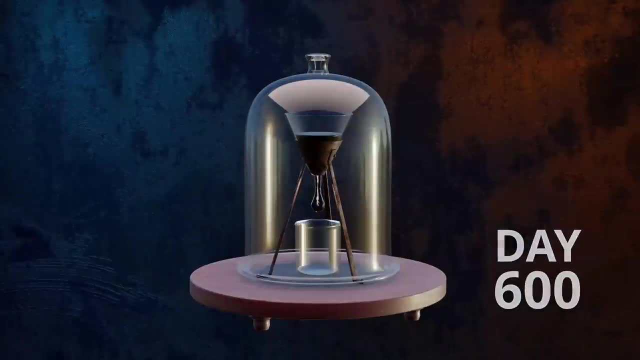 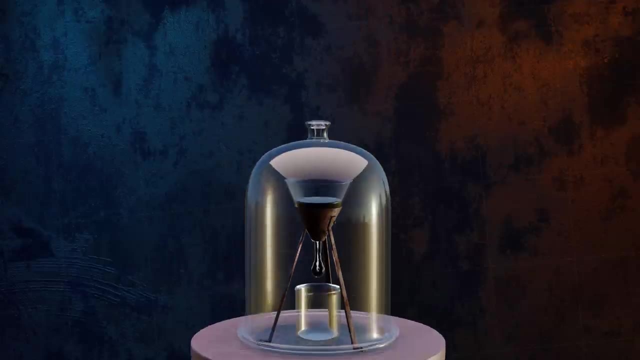 Because of its extremely high viscosity. only 9 drops have fallen into the beaker since then. It is the world's longest running continuous lab experiment. On the other end of the spectrum we have gases which generally have much lower viscosity than liquids. Air has a viscosity of .018 centipoise at room temperature, for example. 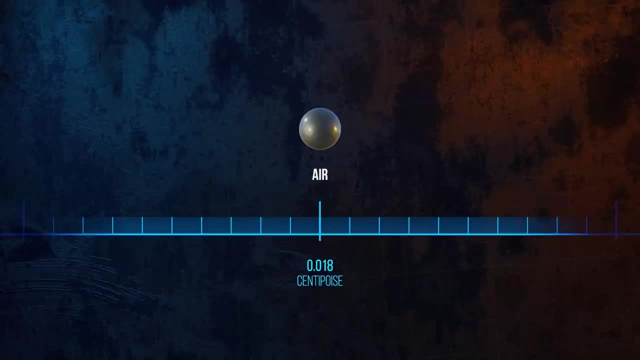 One very interesting substance is helium-4,, the common isotope of helium A gas. under normal conditions it becomes a liquid when cooled to below 4 kelvin, and at these low temperatures researchers have found that it can behave like it has zero viscosity. 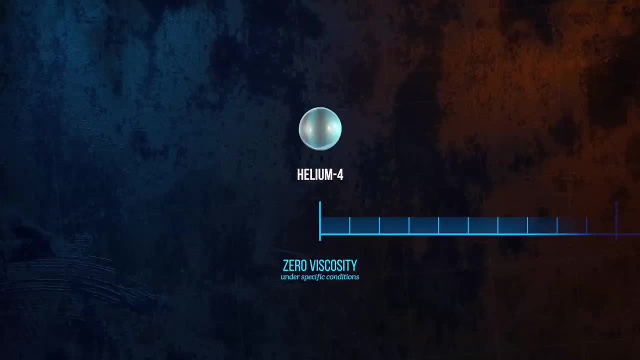 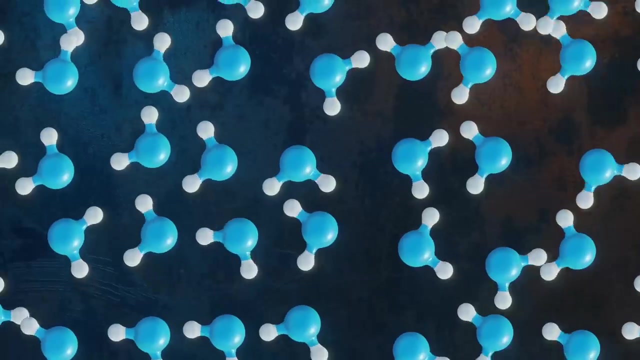 Substances that behave in this way are called superfluids. So we know how to define viscosity, but what actually causes it on the molecular level? In liquids, viscosity is caused by intermolecular cohesive forces which bond layers of the fluid together. 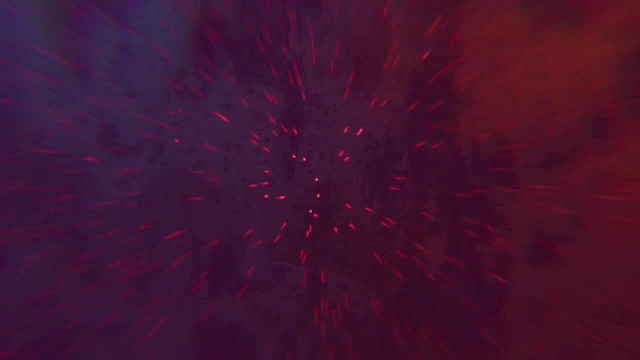 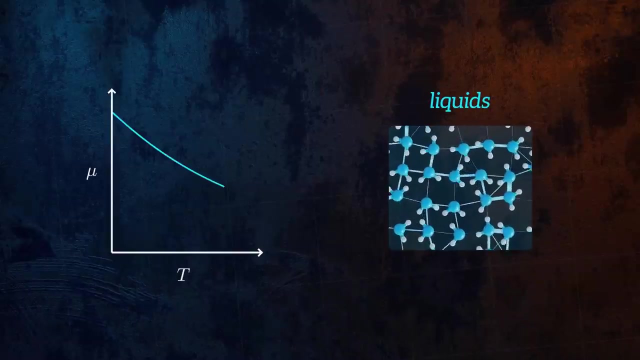 And in gases it's caused by intermolecular collisions which create interaction between adjacent layers of the fluid. Viscosity is highly dependent on temperature. In liquids, it decreases as temperature increases. This is because, at the molecular level, an increased temperature allows molecules to 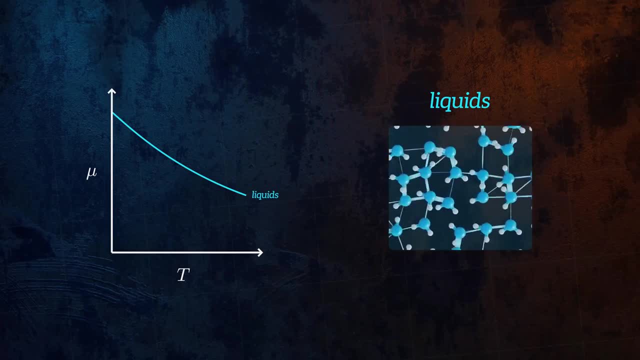 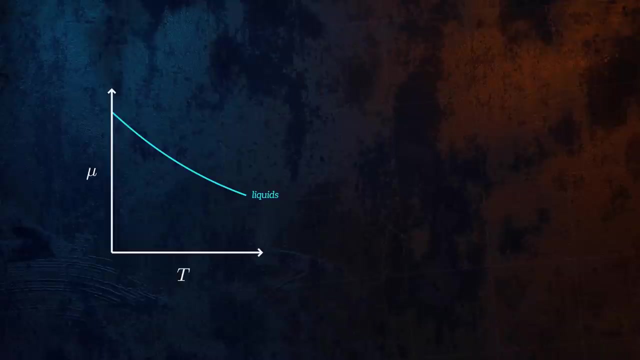 more easily escape the attractive forces of the adjacent molecules. The viscosity of water, for example, reduces from 1 centipoise at 20 degrees Celsius to 0.5 centipoise at 50 degrees Celsius. But temperature has the opposite effect. in gases, Viscosity increases with increasing temperature. 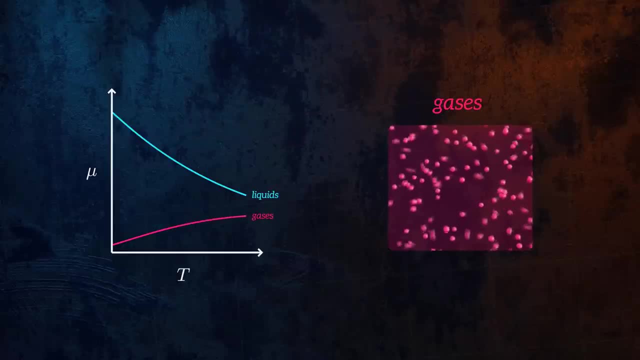 because the higher temperature means that gas molecules have more random molecules. So the more the gas molecules are in contact with each other, the more the gas molecules are in contact with each other, The more the gas molecules are in contact with the other. 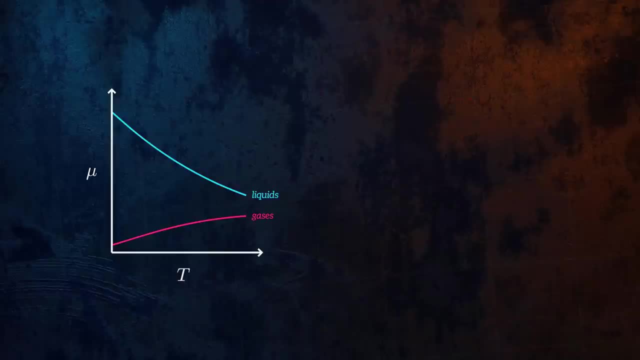 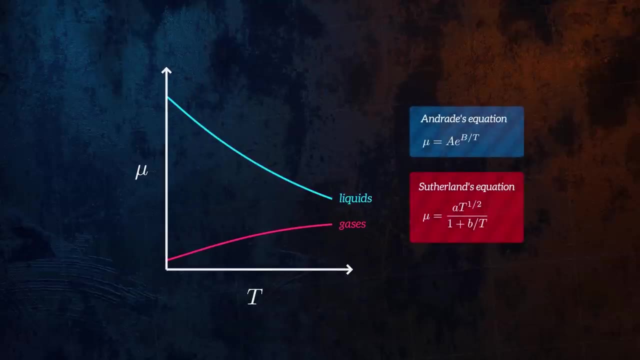 the more the gas molecules are in contact with the other. The temperature dependence of viscosity can be modeled using simple empirical correlations. We can use Andrade's equation for liquids and Sutherland's equation for gases, where the various constants are determined for each fluid by experimentation. 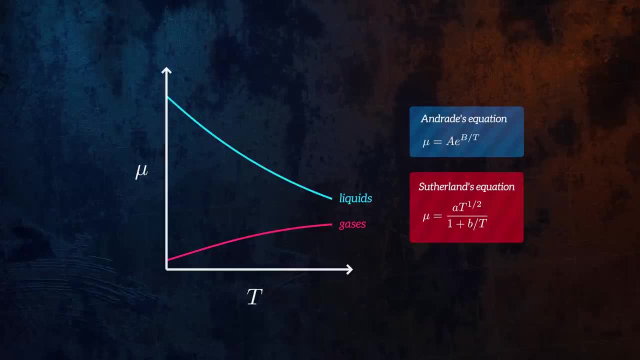 Viscosity also varies with pressure, although to a much lesser extent than temperature, and so pressure dependence is often neglected, Because it fundamentally affects how fluids behave. viscosity is a very important parameter in fluid mechanics. It appears in the equation for Reynolds number, for example. 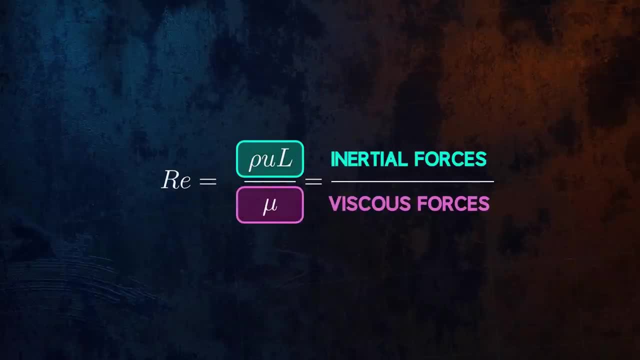 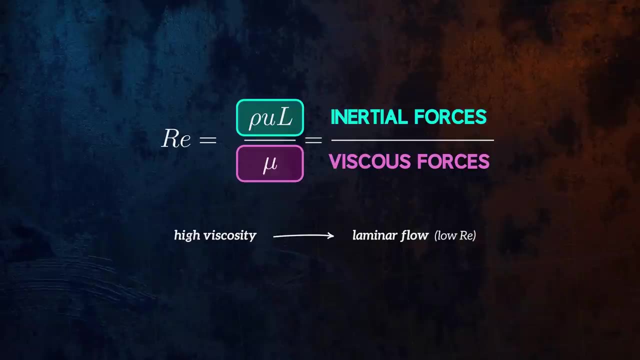 and so affects whether flow is likely to be laminar or turbulent. Flow of high viscosity fluids is more likely to be laminar because any small turbulent disturbances are more easily dampened out by the larger shear stresses. Viscosity also causes the pressure drop along the flow. 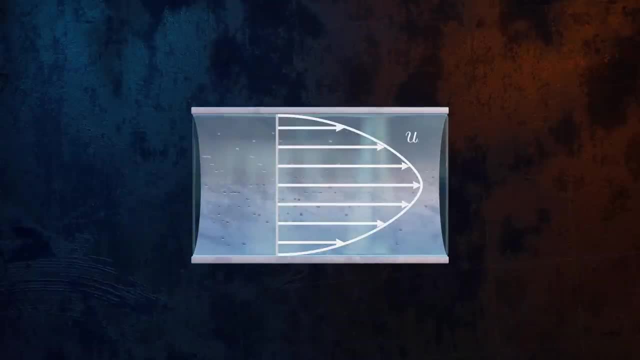 Without viscosity, there would be no shear stresses imparted by the pipe wall, and the velocity profile would look like this: The existence of viscosity can make modeling flow quite complicated, and so engineers often try to neglect viscous forces where possible. The assumption that viscous forces are negligible is typically only applied to certain regions. 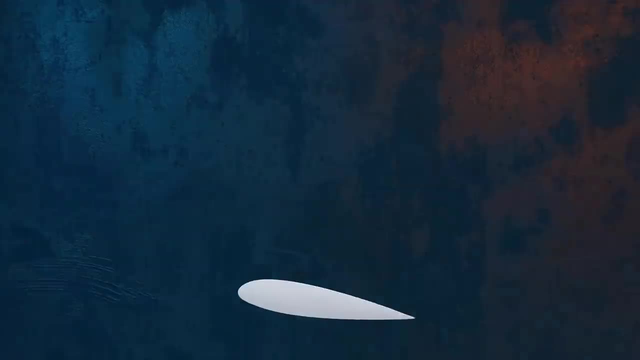 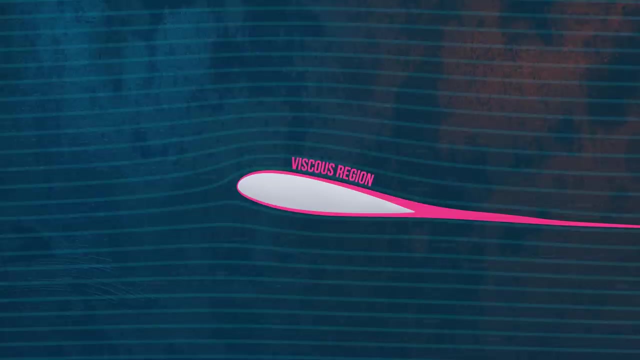 within a larger flow system, It's never valid for flow. For example, if you have a flow close to a boundary, where viscous forces are always significant, But outside of the boundary layer, at high Reynolds numbers, viscous forces can often be neglected. 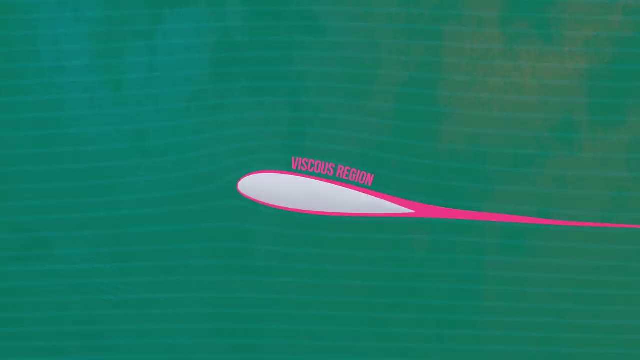 Flow where viscous forces can be neglected is said to be inviscid. Assuming that the flow is inviscid doesn't mean we're assuming the fluid has no viscosity. It just means that we're neglecting viscous forces because they're small compared to other forces. 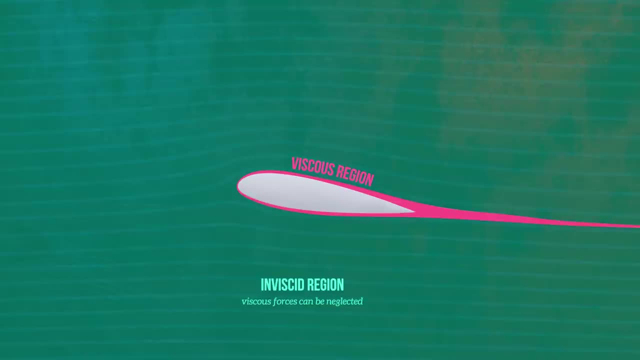 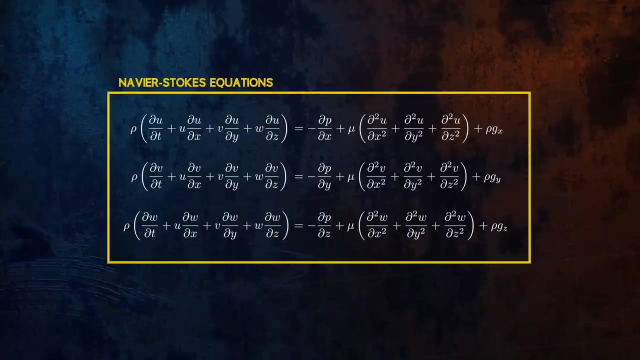 Doing this makes analysis of the flow much easier. The Navier-Stokes equations define the behavior of fluids but are very difficult to solve. Assuming that flow is inviscid means that we can neglect the viscous terms which contain the higher order derivatives. 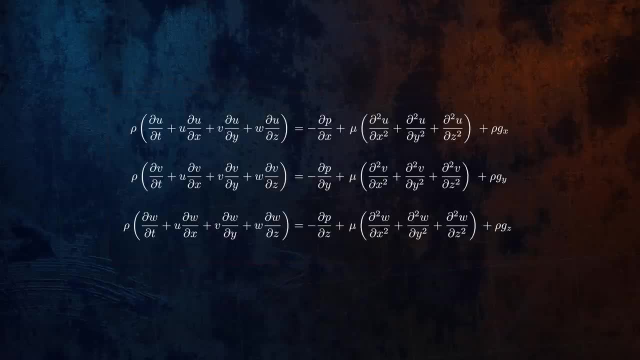 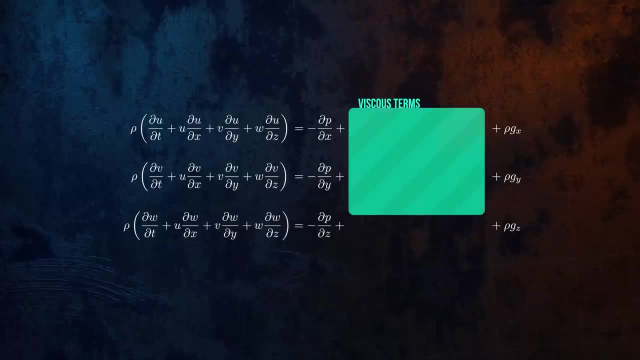 The resulting equations for inviscid flow are called the Euler equations, and they're much easier to solve. Inviscid flow is also a key assumption in the theory of flow, but it's not always the case that flow is inviscid. 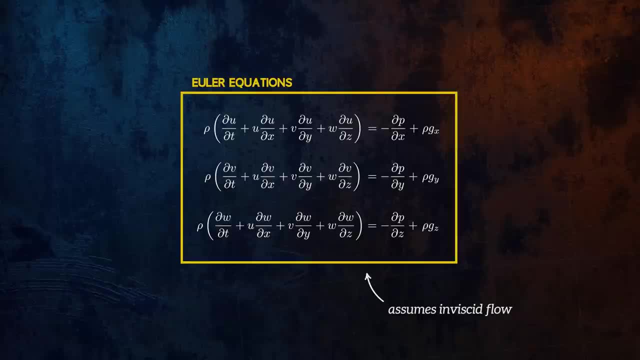 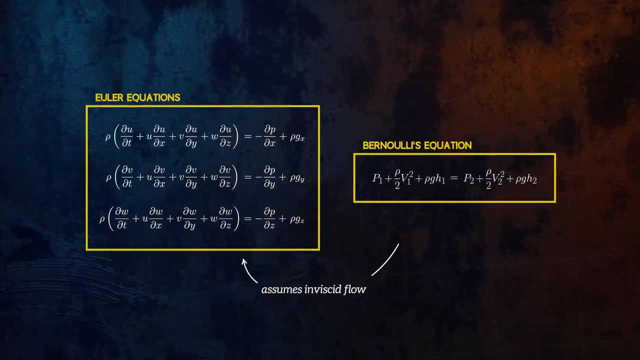 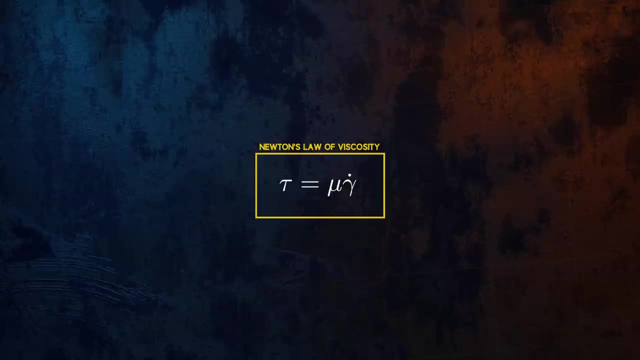 In the theory of flow. the flow is not always the same. The flow is always the same. The flow is always the same. Inviscid flow is also a key assumption in the derivation of Bernoulli's equation. We said earlier that fluids that obey Newton's law of viscosity are said to be Newtonian. 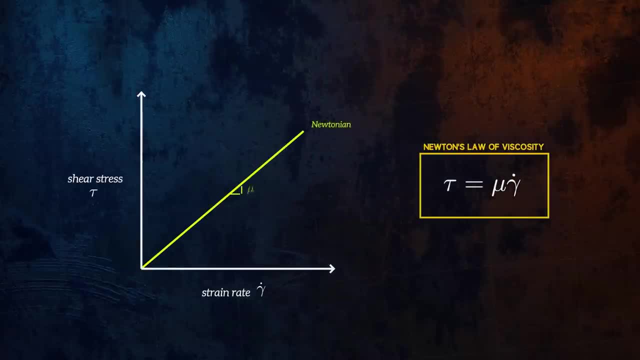 The shear stress increases linearly with the strain rate, But for some fluids the relationship between shear stress and strain rate is non-linear. These are called non-Newtonian fluids and there are two main types: shear thickening fluids and shear thinning fluids. 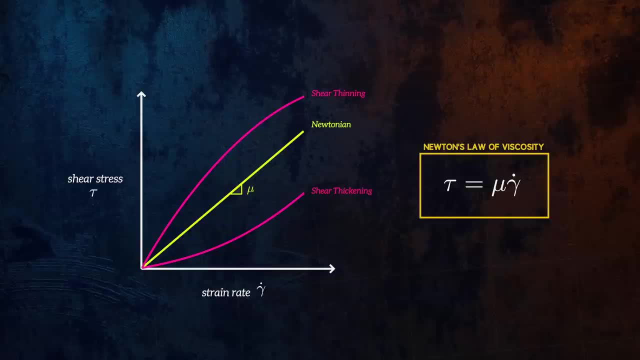 For shear thickening fluids, the apparent viscosity increases as the strain rate increases, And for shear thinning fluids, the apparent viscosity reduces as the strain rate increases. Paint is an example of a shear thinning fluid. It's easily applied with a brush, but doesn't drip from the wall once it has been applied. 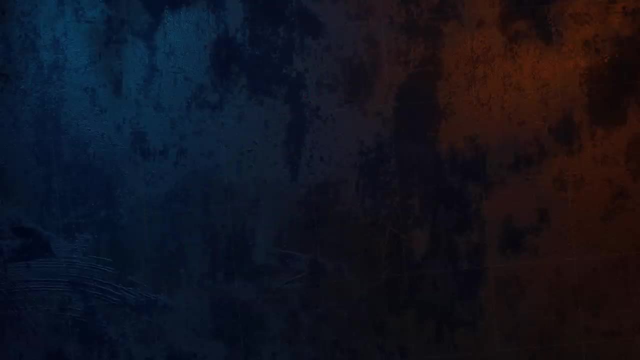 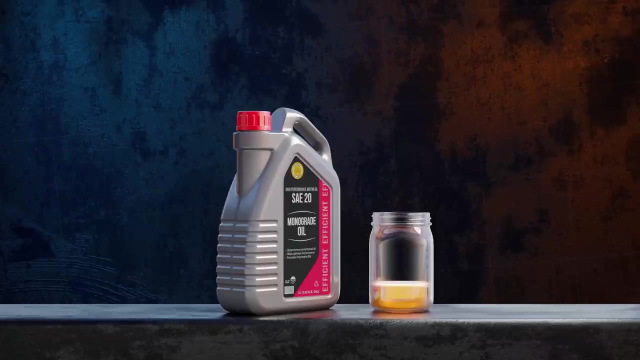 It's a fundamental parameter in the study of fluids. Engine oil is one example of an application where viscosity and the effect of temperature play crucial roles. I've included a bit more discussion about engine oil viscosity in the extended version of this video over on Nebula. 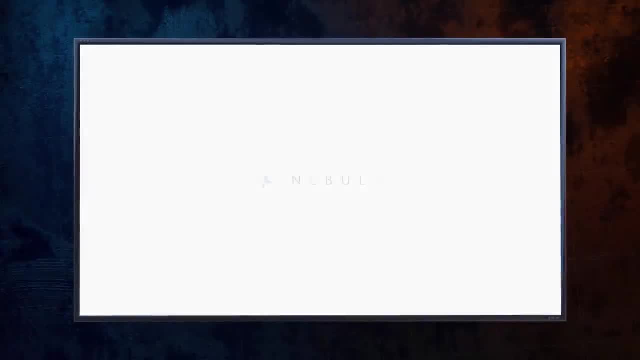 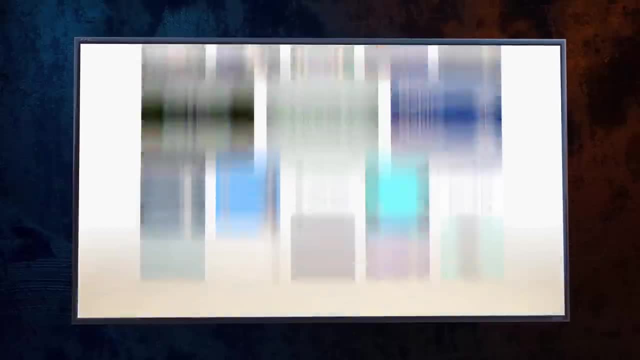 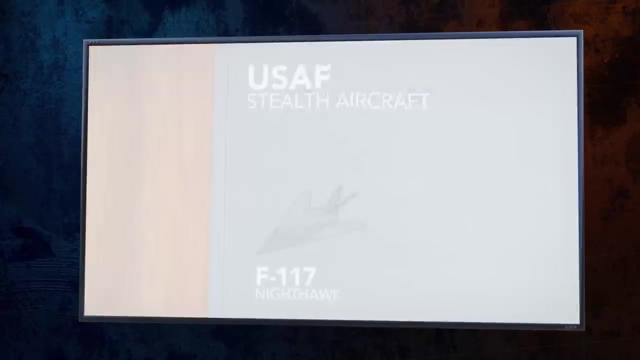 Nebula is a streaming platform built by independent educational creators. It's a place where you can find loads of amazing original content, like Mustard's The Origins of Stealth, that explores the history of the F-117 Nighthawk, But it also has extended versions of videos from your favorite creators. 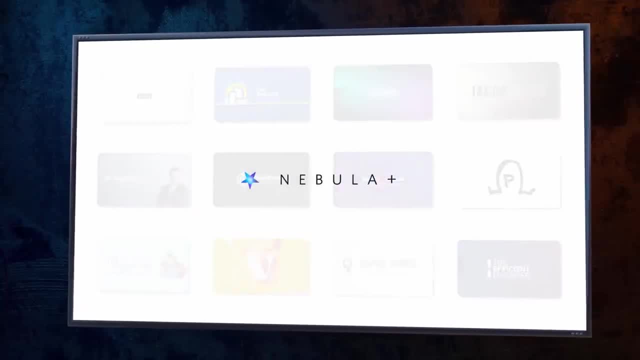 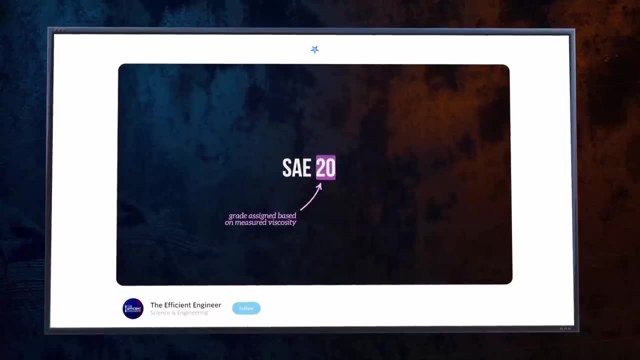 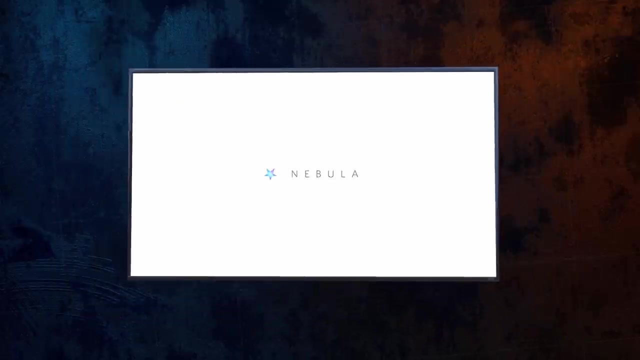 with what we're calling Nebula Plus. The Nebula Plus version of this video includes a few extra minutes on engine oil viscosity, and that content replaces this sponsor segment, since Nebula is completely ad-free. To make Nebula even better, we've teamed up with CuriosityStream.